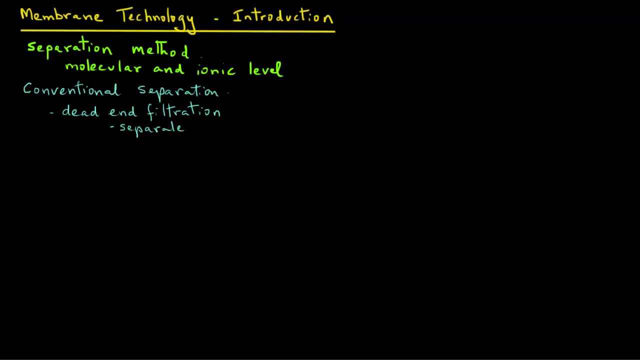 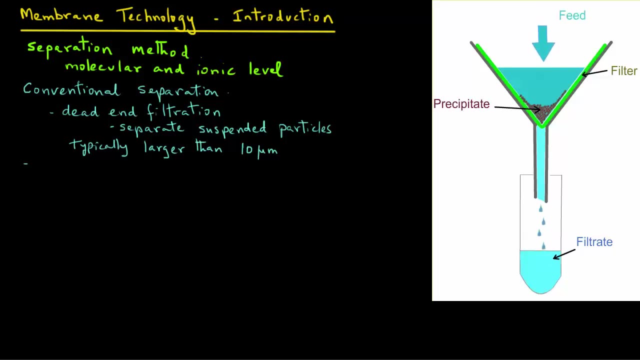 where we may use filtration to separate suspended particles that are typically larger than 10 micrometers. A very common procedure will be where particles are retained by a filter and those particles start to build up with time as what is called a cake layer. that results in increased resistance to filtration. 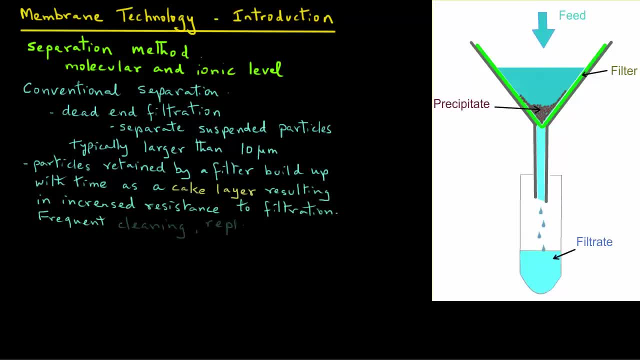 So it requires frequent cleaning and also, of course, replacement of filters. Now, in this type of a system, gravity is the main force. gravity is the main force for separation And, as we note here, the feed flows in a perpendicular direction. 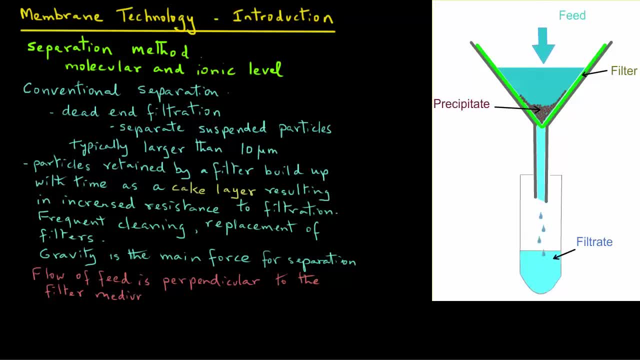 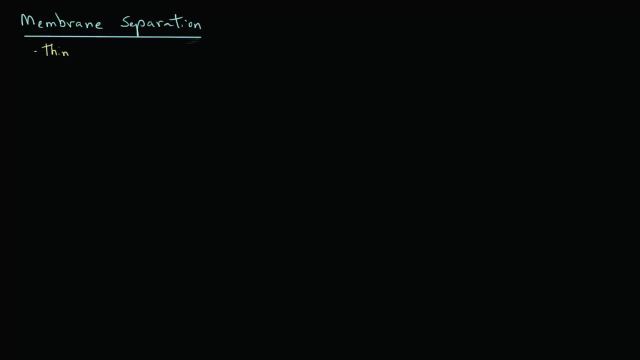 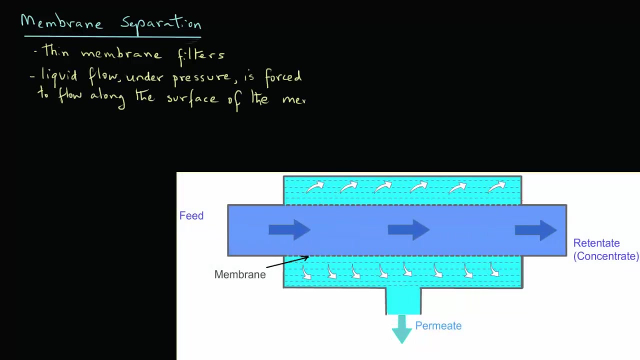 to the filter medium. Another feature to note in the conventional separation system is that it's open to the atmosphere. Next we will look at membrane separation systems, where the filters that are used are very thin membrane filters. The liquid flows under pressure and it is forced to flow along the surface of the membrane. 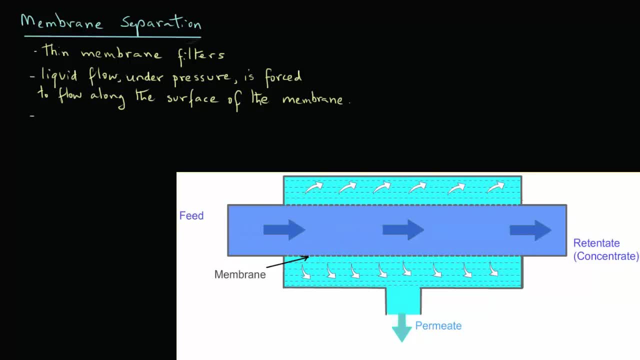 This is in contrast to the dead-end filtration that we just saw, where the flow was in a perpendicular direction to the surface of the filter. The flow then sweeps the particles that get retained. The flow then sweeps the particles that get retained. The flow then sweeps the particles that get retained. 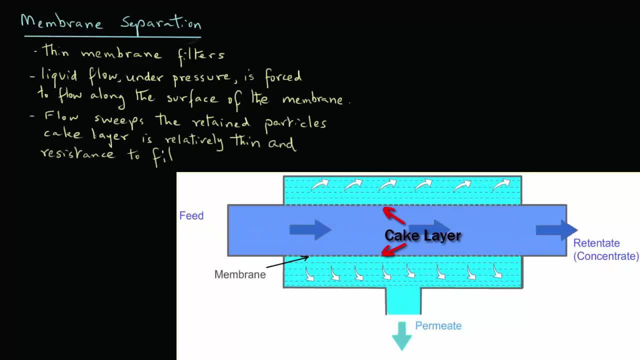 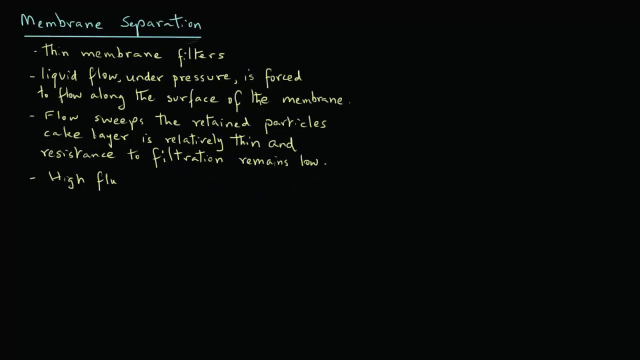 as a cake layer And the cake layer remains relatively thin And therefore the resistance to filtration remains low in comparison, again, to the dead-end filtration. So in membrane filtration because of the flow of the liquid there is a high flux that is maintained. 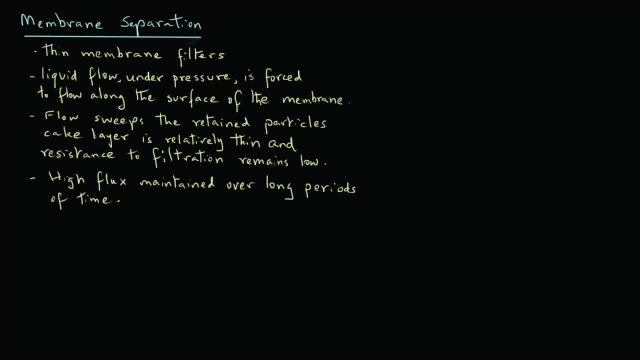 over a long period of time. Recall that the flux is the permeate that is flowing through the membrane. In contrast to dead-end filtration, the membrane separation systems are closed systems. They are not open to the atmosphere And the particle size that is separated.